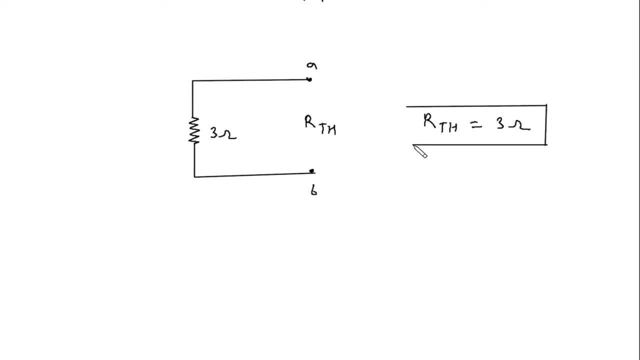 Now we have to find Vth. we have to find Vth, Vth, so this will be Vth. now to find Vth. let's convert this 18 volt into its equivalent current source using source transformation, So this will be 6 ohm parallel with current source. 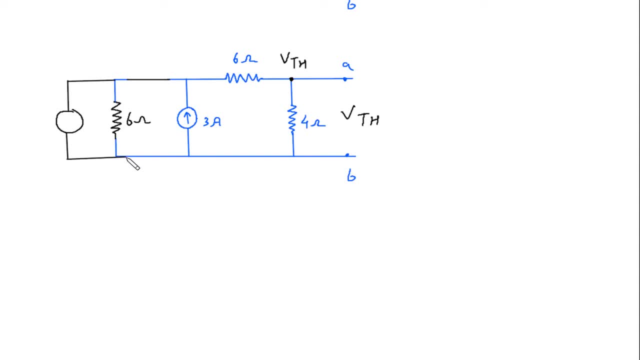 The direction of current source will be upwards. now this will be 18 by 6, so 18 by 6 will be 3 Ampere. so this will be 3 Ampere, So this will be 3 Ampere. current source voltage upon resistance is equal to current. 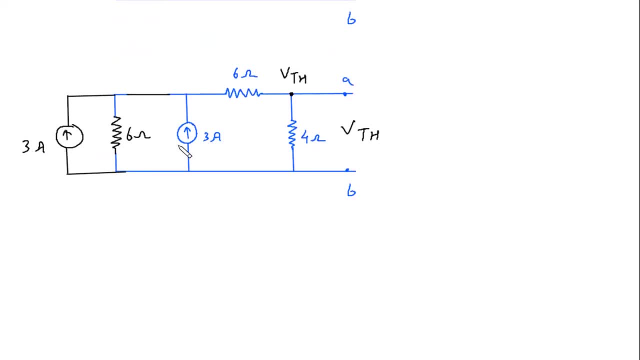 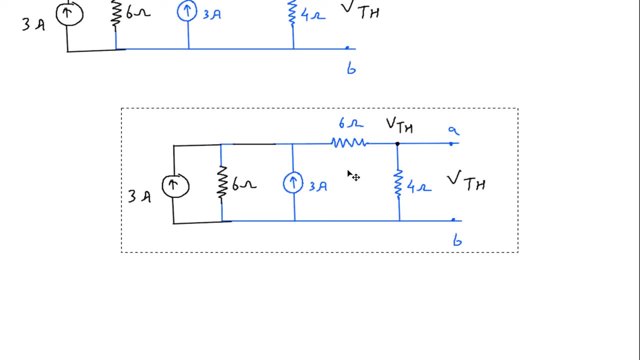 Now, as we can see that this 3 Ampere and 3 Ampere are in same direction, so this will get added. So this will be 3 plus 3, 6 Ampere. So this will be 3 plus 3, 6 Ampere. 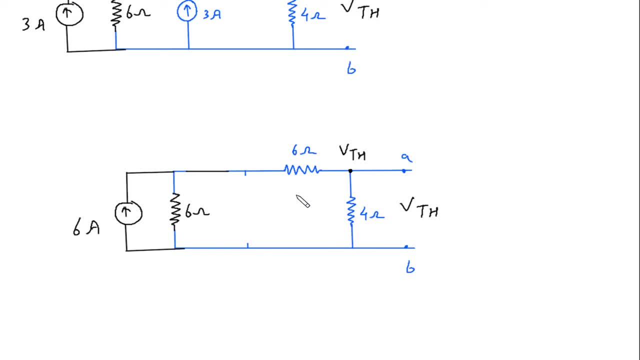 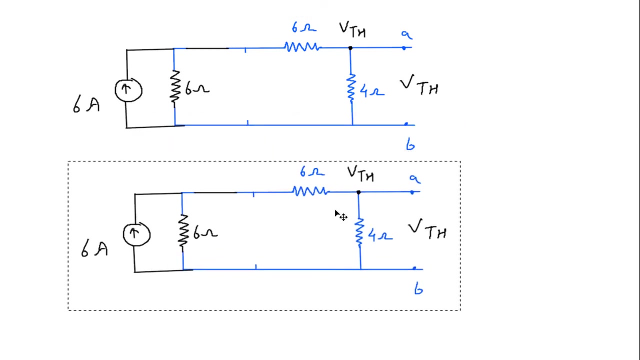 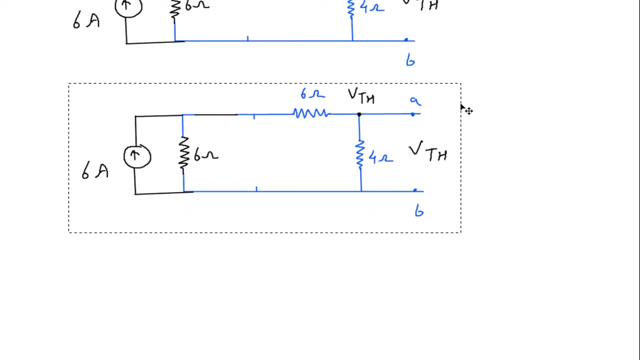 Now again, we will convert this current source into its equivalent voltage source, so this will be 3. 6 ohm and here voltage source. this is 6 ohm. this is voltage source. This will be current. into resistance- Current is 6 Ampere- into resistance is 6 ohm. 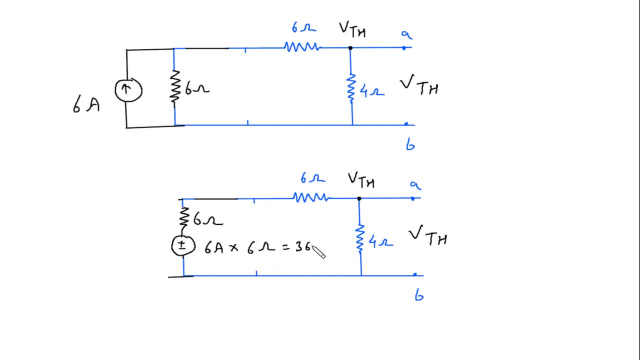 So this is the current source. Current of Free heated water with resistance is 6 Ampere per Kelvin, So this will be 36 volt, 36 volt, 36 volt. Now we have to find current through this resistor, 4 ohm. 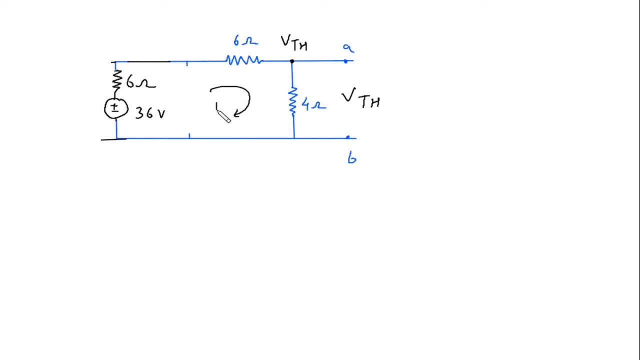 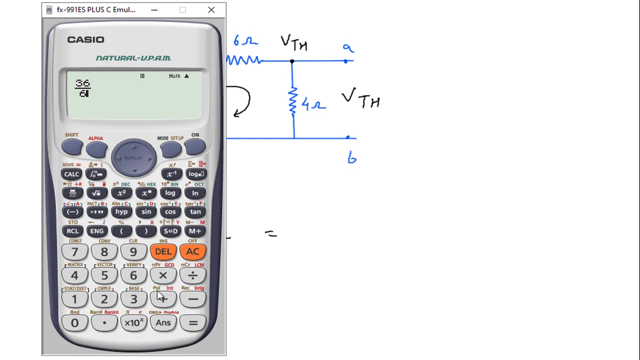 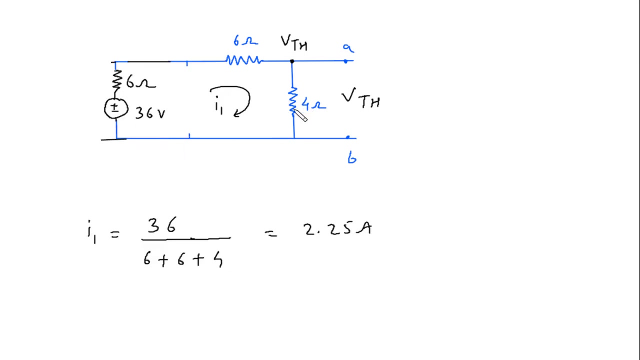 So this will be- let's assume this is current I I1.. So I1 is equal to 36 by 6 plus 6 plus 4.. So this will be 36 by 6 plus 6 plus 4, 2.25, 2.25 Ampere. 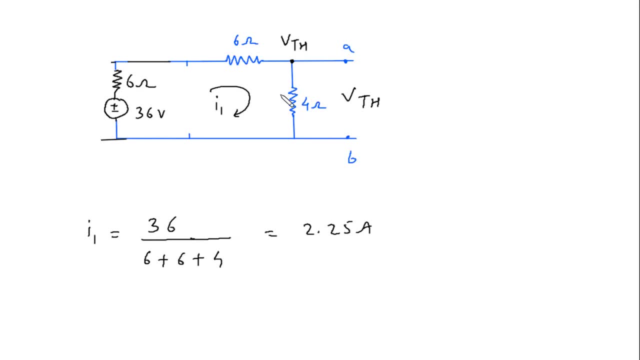 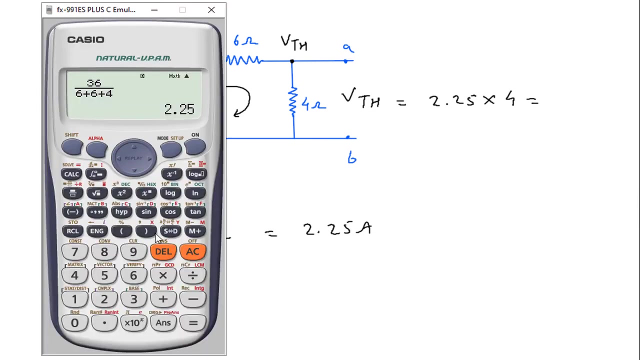 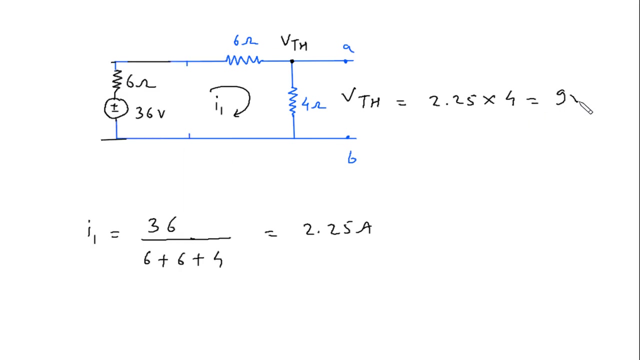 So from this we can find the value of Vth, So Vth will be Vth. Vth is equal to current 2.25 into resistance is 4 ohm, So 2.25 into 4.. This is 9 volt. 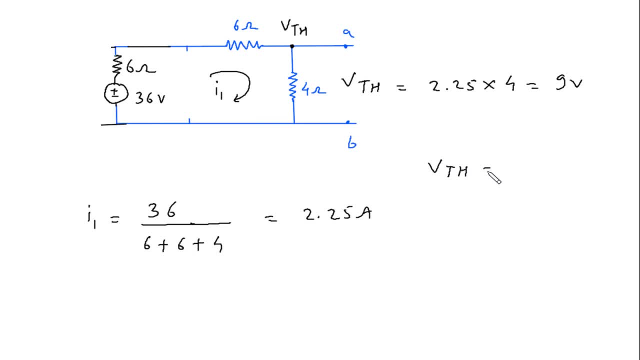 So therefore Vth is equal to 9 volt. Now we have the value of Rth, which is 3 ohm, and Vth. Now we will draw equivalence equivalent. So this is Rth And this is Vth plus minus. 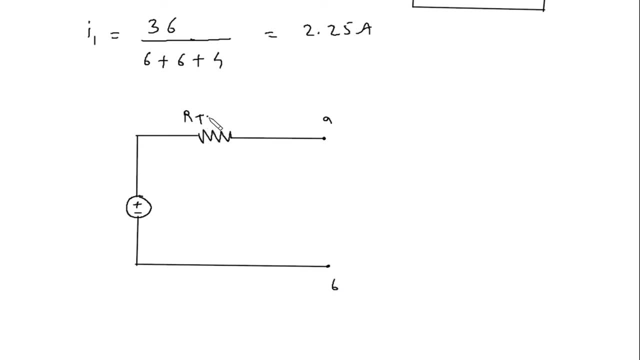 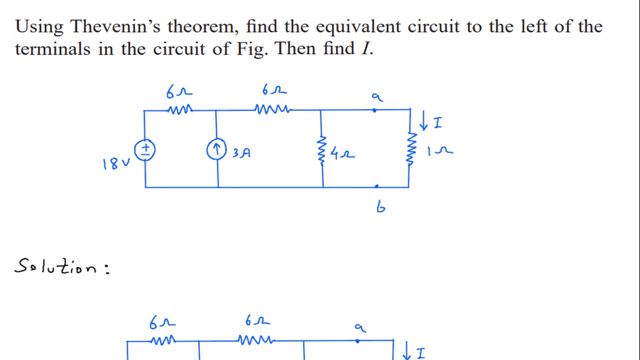 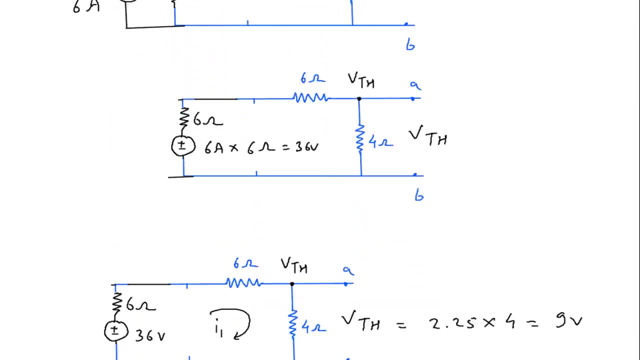 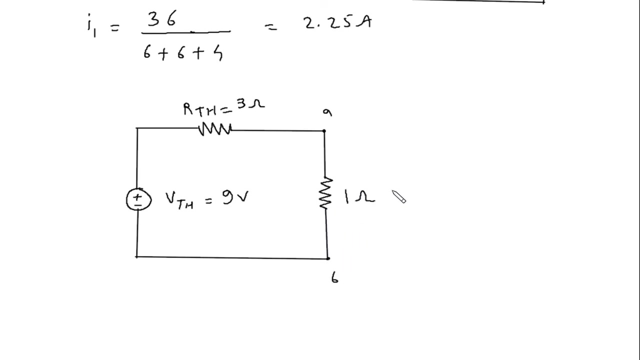 This is A. this is B. this is Rth is equal to 3 ohm. This is Vth: Vth is equal to 9 volt. Now we have to find this: I and this RL is 1 ohm. This is RL, which is 1 ohm. 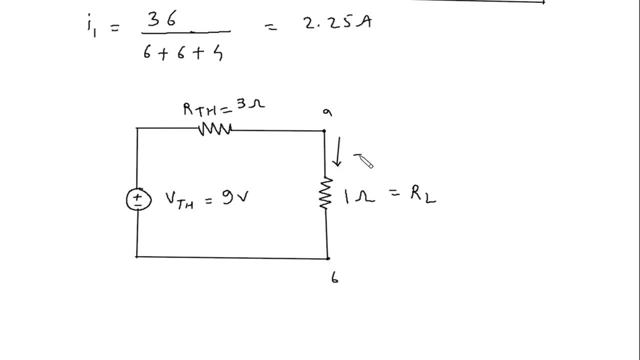 This is RL. this is current I. This is equal to IL. This is current I. This is equal to IL. This is current I. This is current I. This is 1 ohm. This is Rth линke.